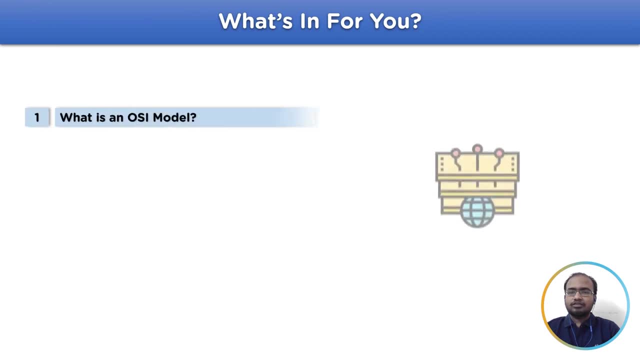 further ado, let us begin with the plan for today's topic. First we will have a quick recap on the OSI model. Then we will dive into our core topic, the network layer. Moving on, we will have a detailed understanding for the major functions of network. 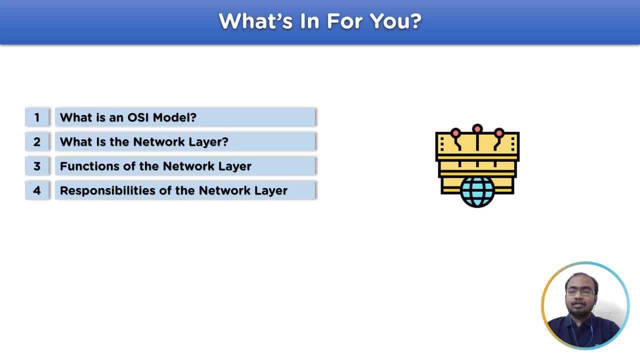 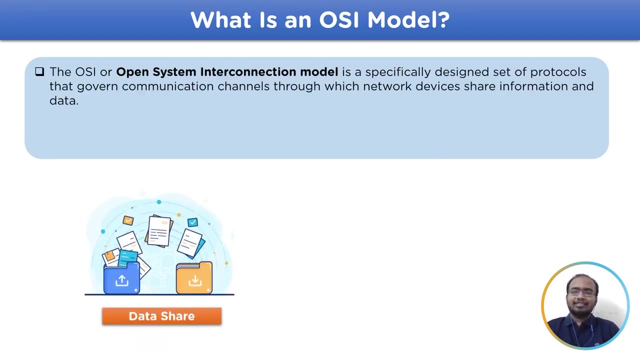 layer. Finally, we will wrap up this session with a discussion on the responsibilities of the network layer in the OSI model. Now the OSI model stands in the context for Open System Interconnection Model, a specifically designed set of protocols and standards governing the data modeling and conversion for proper transmission. The OSI 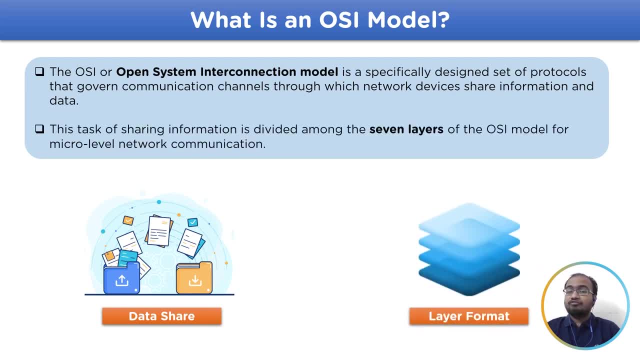 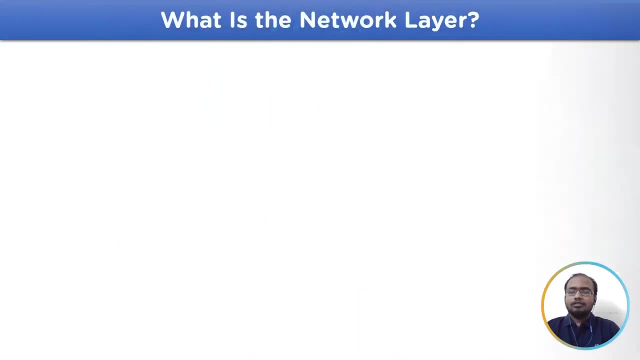 model is divided into seven layers which perform specific functions and apply protocols to maintain data quality without any error. Now let's move on to the core topic for this session: what is network layer? Let's first look at the network layer. The network layer is responsible for breaking. 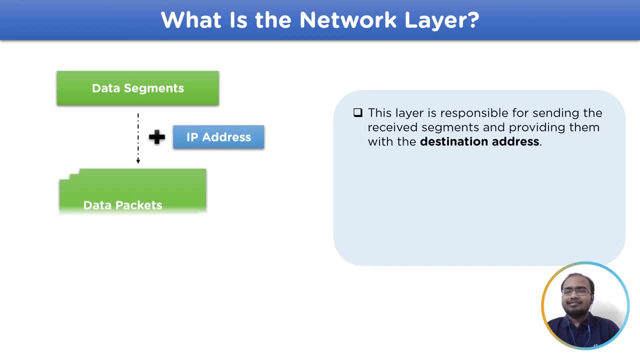 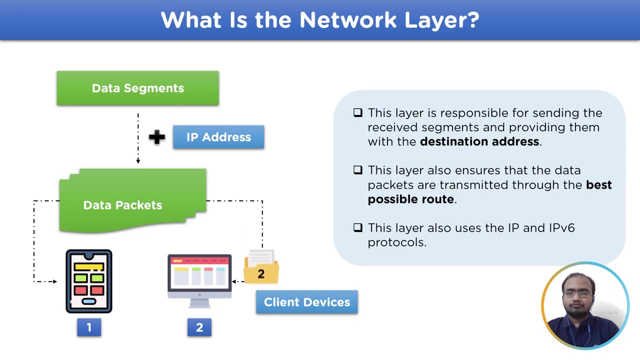 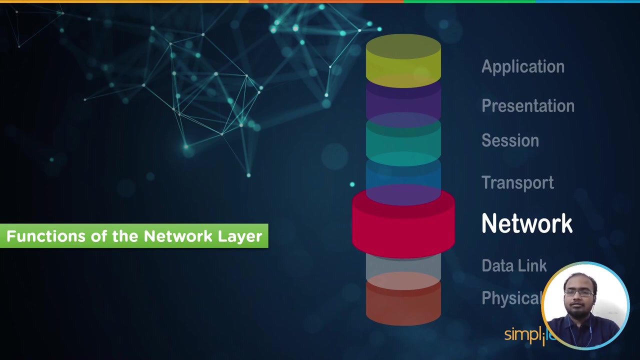 down the segment into data packets and resembling them on the receiving end. This layer also ensures that the packets are transmitted over the best possible route to the destination system governed by the internet protocols. So now, moving forward, let us look at the networks layer function. But before we begin, 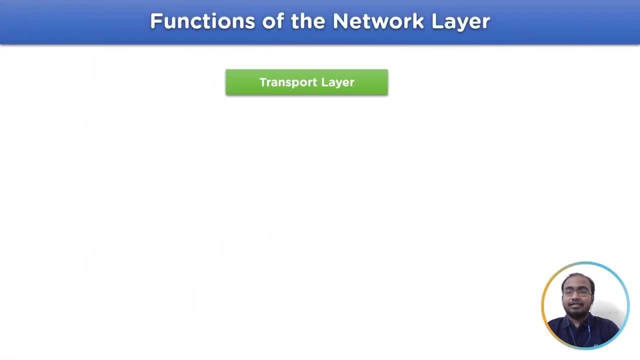 First let's understand the data flow between the network layer and the other layers in the OSI model. That is, to begin with the network layer, we will receive data from the transport layer of the OSI model. The network layer handles these data packets by integrating them with the sources and destination. 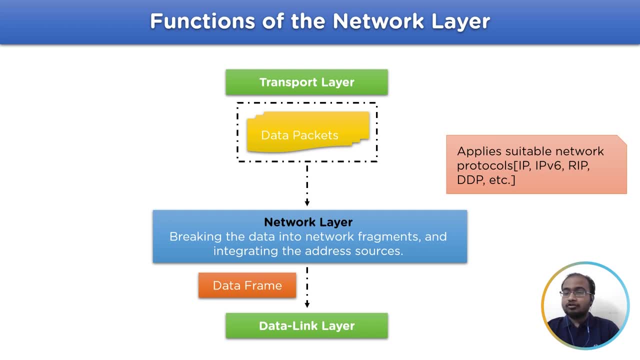 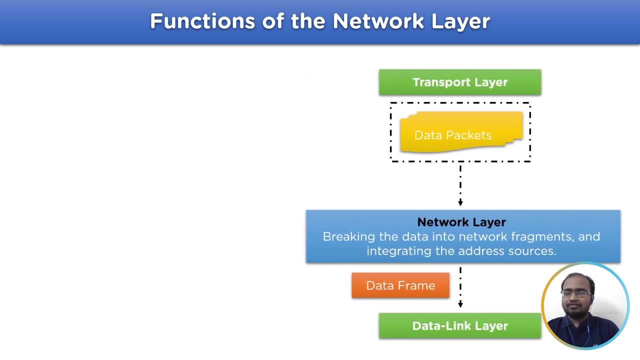 address. It also add network protocol for the proper transmission over the network's channel. Now let's look at the functions of the network layer. First we have inter-networking, that handles the network's channel, as the name suggests. Then we have network addressing, followed by packet routing and packet handling. 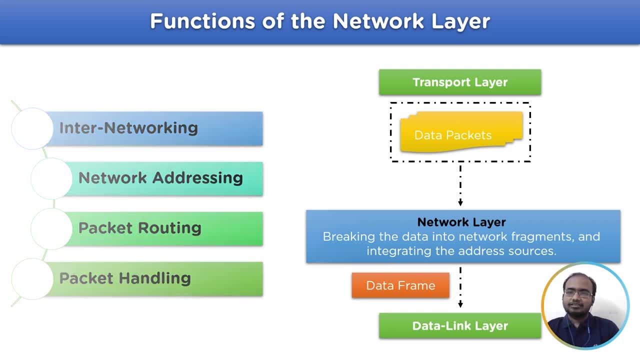 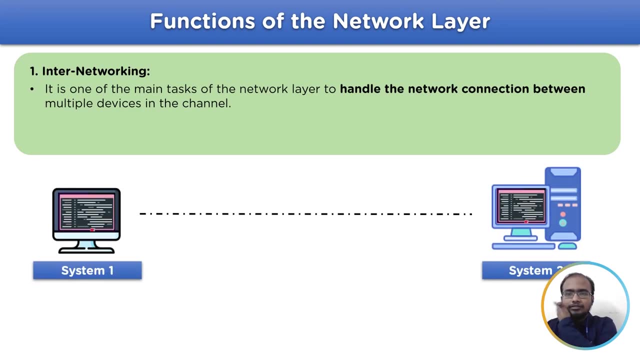 Now let's look at some of the points regarding the functions. First up, inter-networking. it is one of the main task of the network layer to handle the network, The network connection between multiple devices in the channel. This task applies multiple protocols available in the network layer of the OSI model for 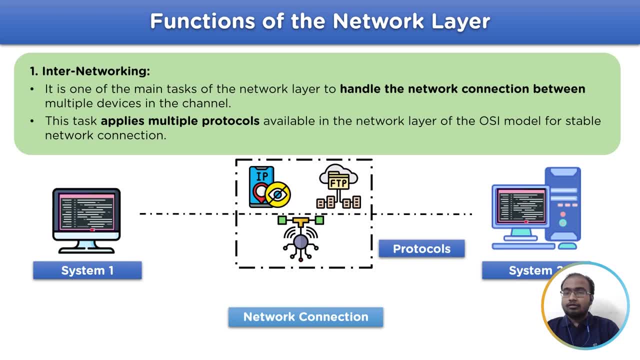 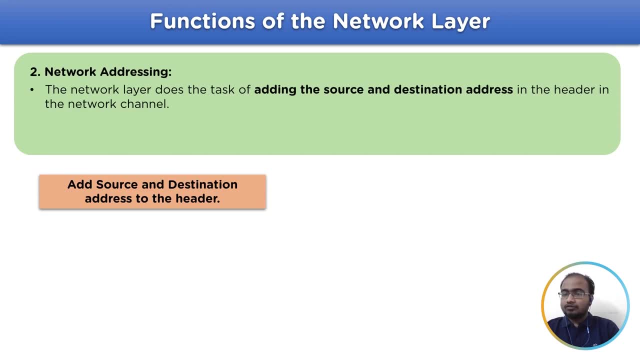 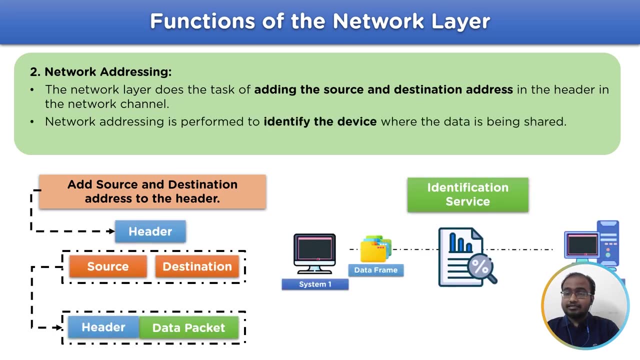 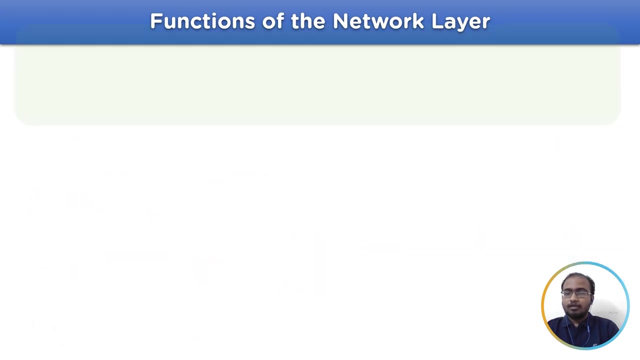 stable network connection. Next up network addressing: The network layer does the task of adding the source and the destination address in the header of the network channel. The network addressing is performed to identify the network. Next up packet routing: Now the establishing and routing path for the data packets is one of the main functions. 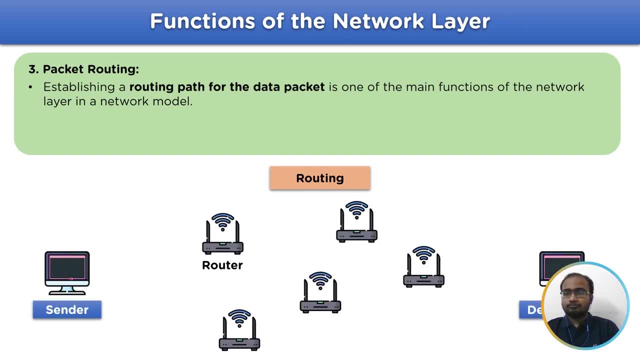 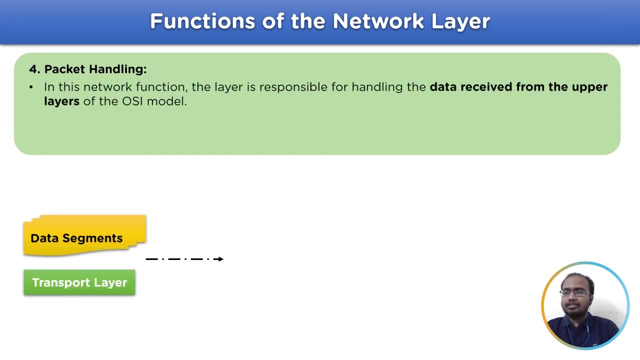 of the network layer. in the network model, A network layer chooses the most suitable path out of the line of the path available in the channel Next up packet handling. In this the network layer is responsible for the network's network, The network function. the layer handles the data received from the upper layers of the 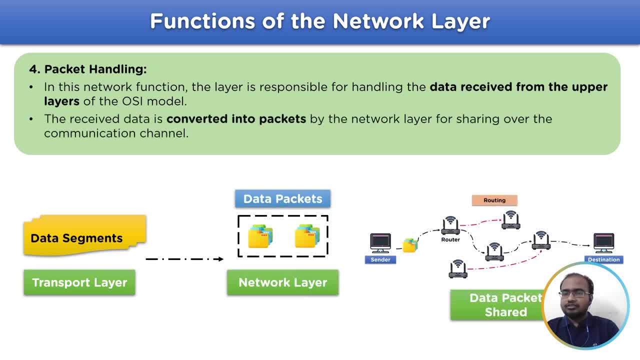 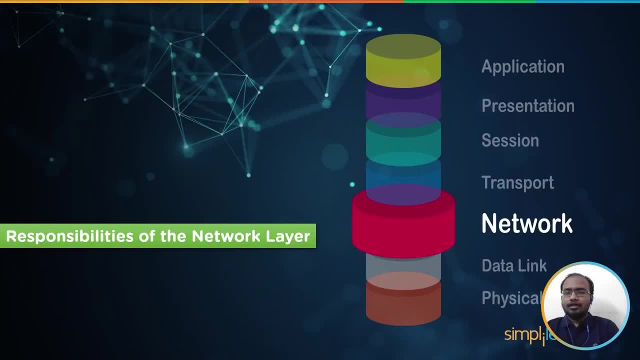 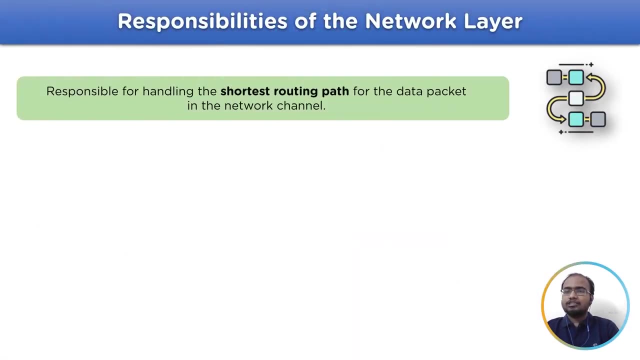 OSI model. The network layer converts the received data into the packets for sharing over the communication channel. Now let's look at the responsibilities of network layer. The network layer is responsible for handling the shortest routing path for a data packet in the network channel. 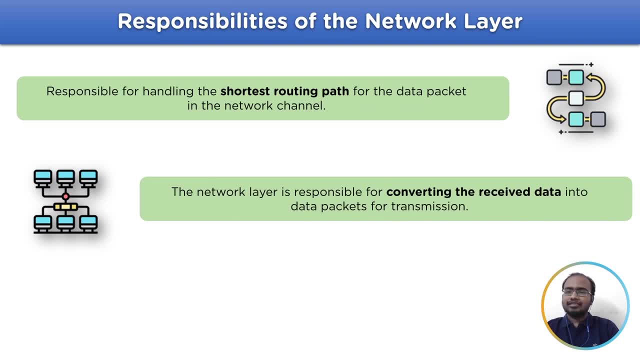 It is also responsible for handling the shortest routing path for a data packet in the network channel. It is also responsible for converting the received data into packets for transmission. This layer also handles the network layer protocol, which is responsible for maintaining the network's traffic in the channel. 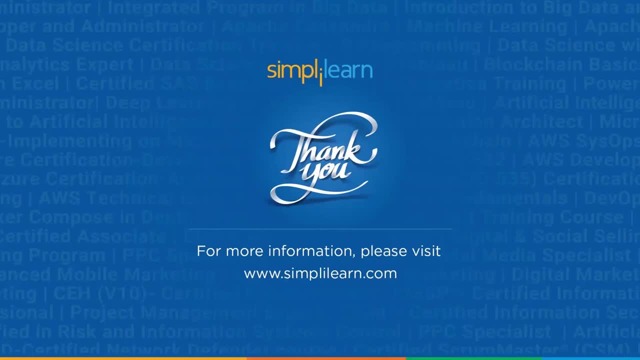 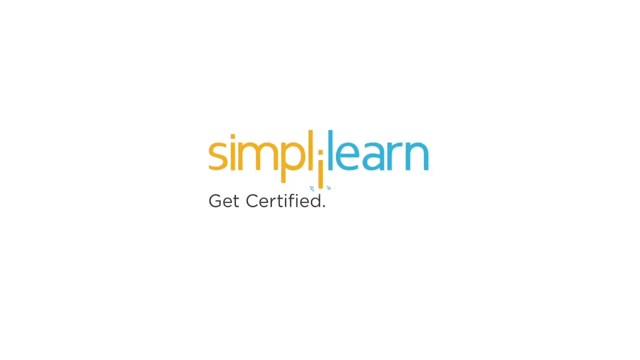 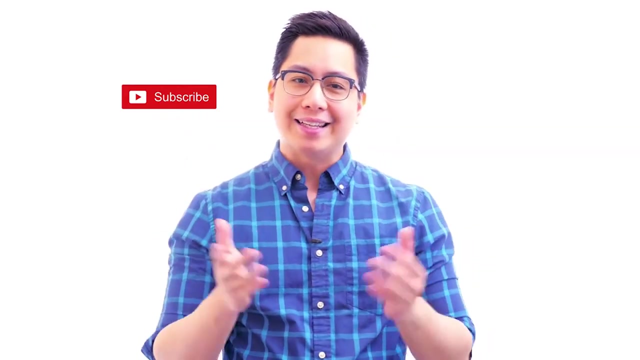 Now, with this, we have covered all the important points related to network layer of the OSI model. If you have any questions regarding this topic, you can ask them in the comment section below. Thanks for watching. Stay safe and keep learning, Hi there. if you liked this video, subscribe to the Simply Learn YouTube channel and click. 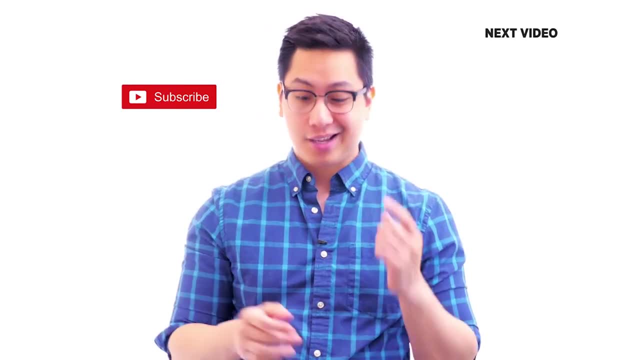 here to watch similar videos. To nerd up and get certified: click here.